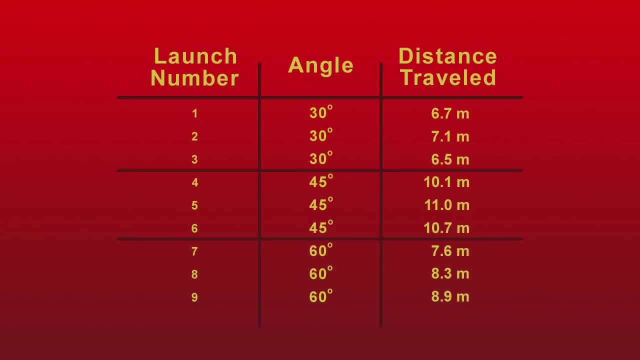 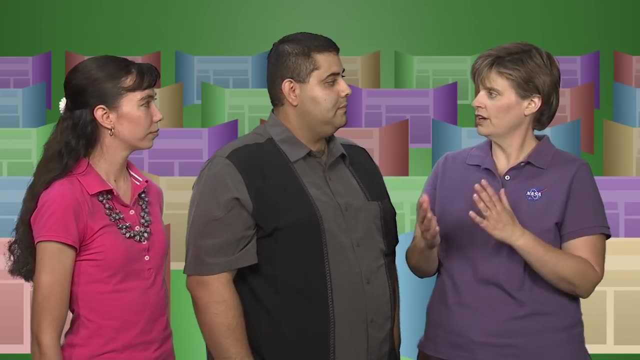 Very good. It sounds like that sort of data would fit nicely in a table and then would also be graphable later. Yes, Obviously there are lots of other variables you could test on in that airplane, but you're not going to, You're just going to set one. 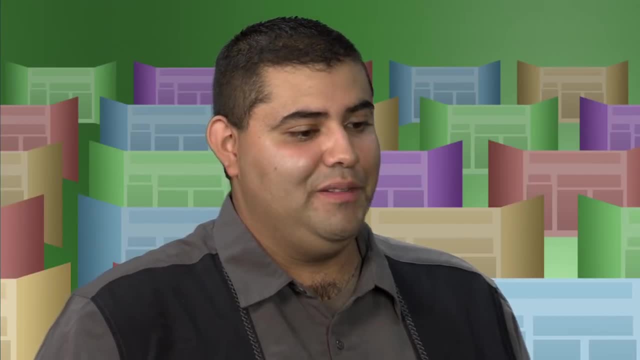 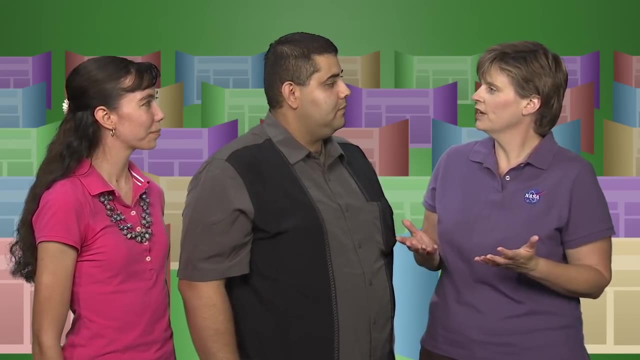 One thing at a time, Correct. Just keep focused and you'll get enough data and you'll be able to make your conclusion on one variable. And if I didn't want to do the launch angle, what else might I change instead? 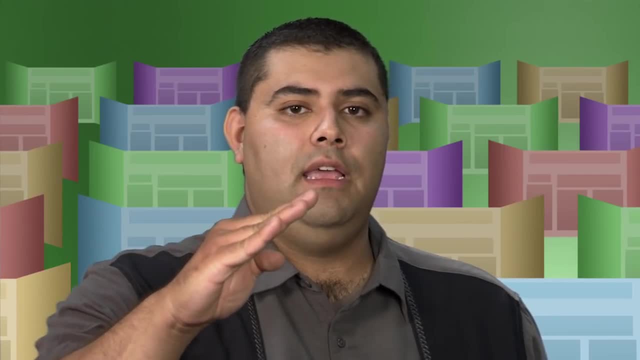 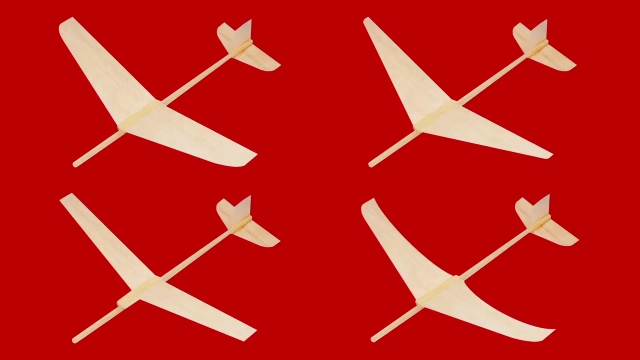 Well, another experiment you could do is keep the angle constant and then change the wing design of your glider. The variable under test is the shape of the wings. So you would do the same procedure for one wing design. You would launch it several times. take your distance measurement. 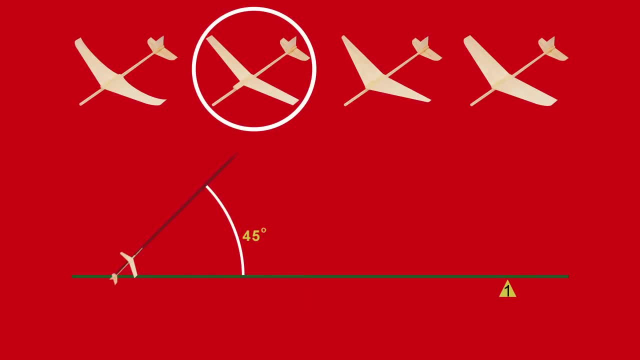 Then you would change your wing design, return to that same angle and do several launches, And you'd do this for as many wing designs as you have. Then you'd compare your distances and find out which one's the best wing design for distance. 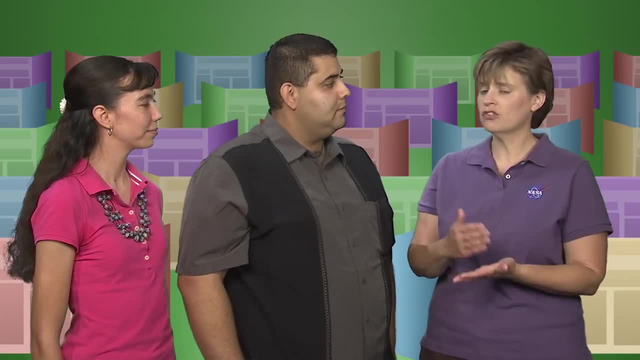 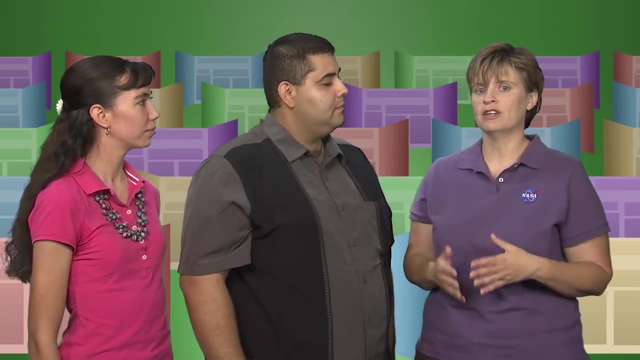 All right, Very good. So which is the best wing design for distance or which is the best launch angle for distance? Both measurable things. We could collect the data in a table, graph it and make a very nice science fair project. 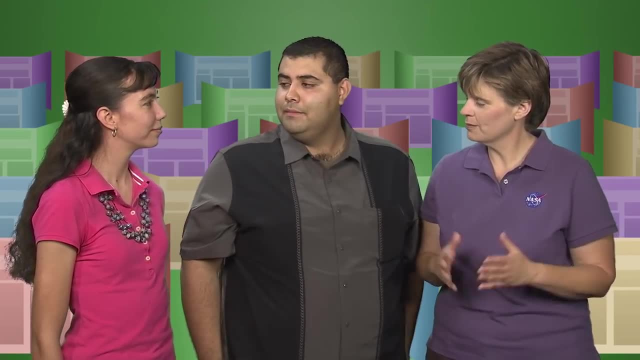 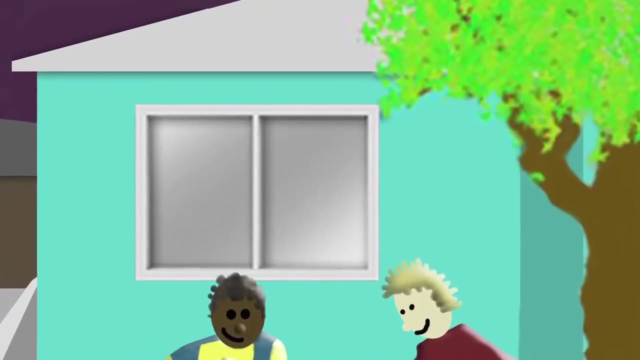 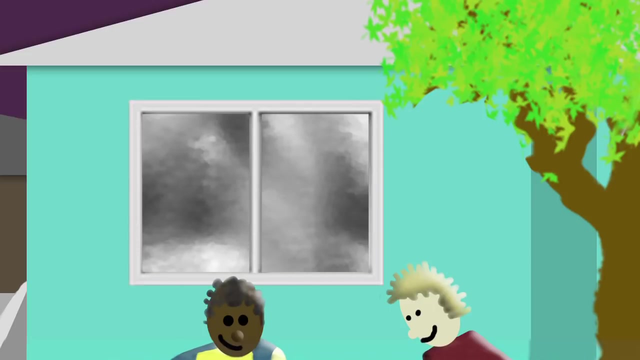 Correct. All right, Serena, do you have another idea from The drawing that you could investigate? Looking at the picture, one science question you could attempt to answer is what type of window covering best keeps a room cool. So you could look at curtains, you could look at blinds- maybe aluminum foil, or even a tree in the yard that's shading that window. 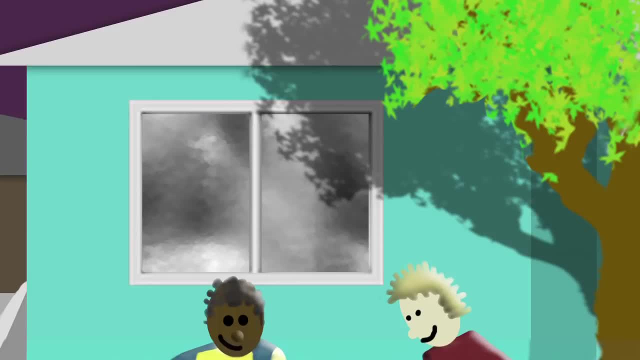 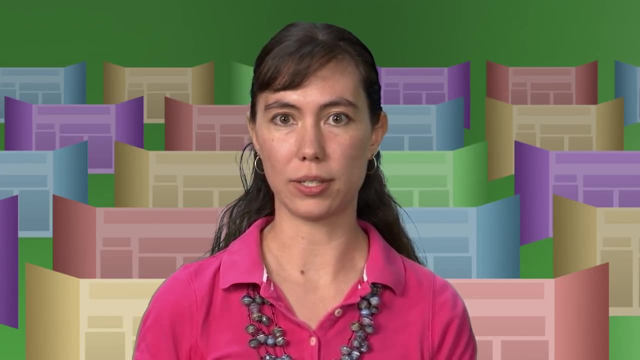 So you would look at those different types of window coverings and measure the temperature within the room at different times during the day and look at the difference between that temperature and the temperature that's outside. Okay, So you, You would be comparing the different coverings. 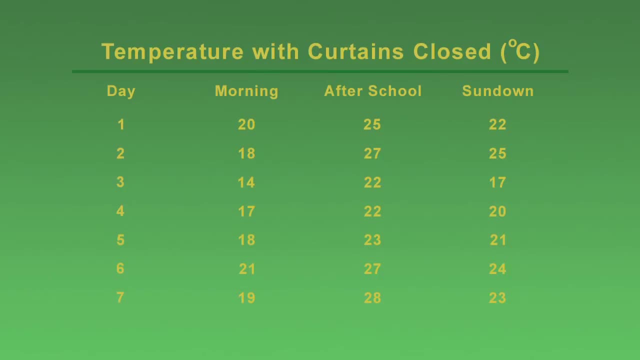 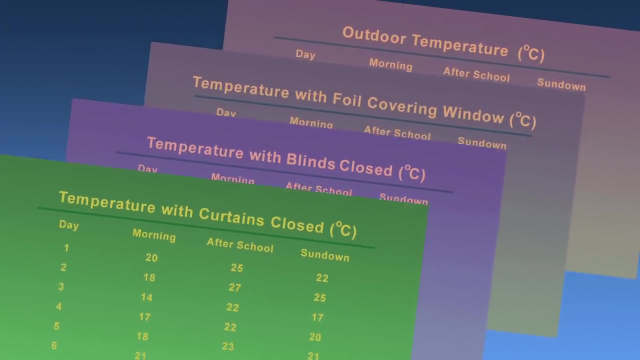 You would investigate the data in the morning, and perhaps after school, when you got home, and then just before sundown. Yes, Make sure you have data from different times of the day, Make sure that everything else is kept the same and the only thing you're changing is the window covering. 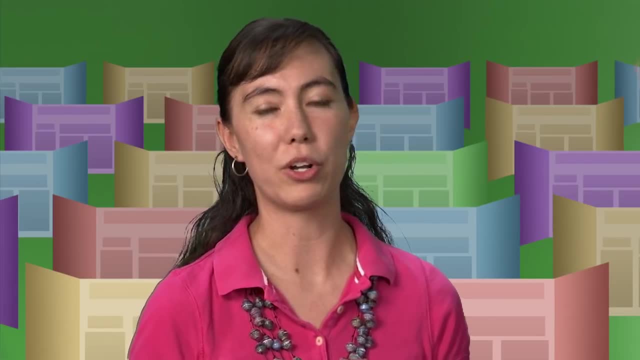 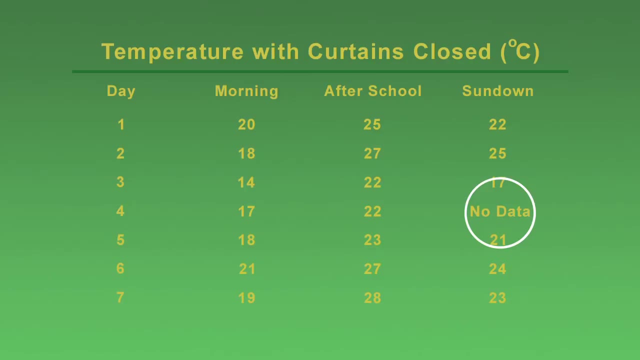 And as many days as you possibly can. One day the thermometer maybe isn't working and you want to make sure that you notice that difference and that you can take that set of data out when you look at the overall trend And possibly cloudy day versus sunny day if that might affect your data.